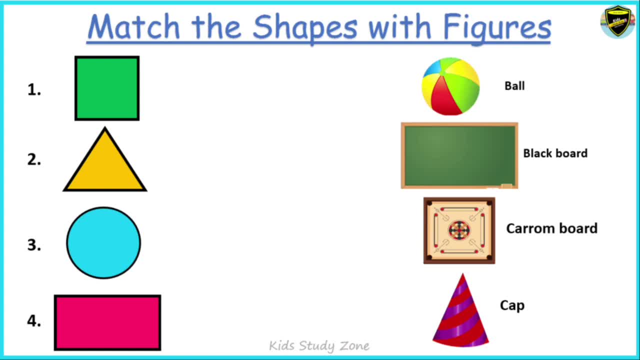 learned today. Now let's do a fun activity to understand the concept better. On the left side you have the shapes we learned today, and on the right side you have some figures. We need to match these shapes with the figure. So let's see the first shape. First one is a square. Now let us 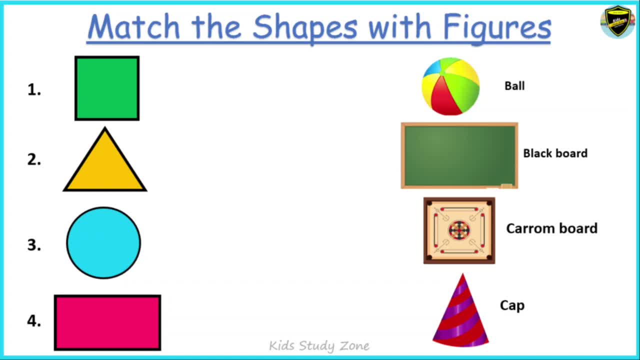 see the options we have on the right hand side. First one is a ball, Second one is a blackboard, Third one is a carom board and fourth one is a cap. Let us see the shape square matches. with which figure Is it a ball? 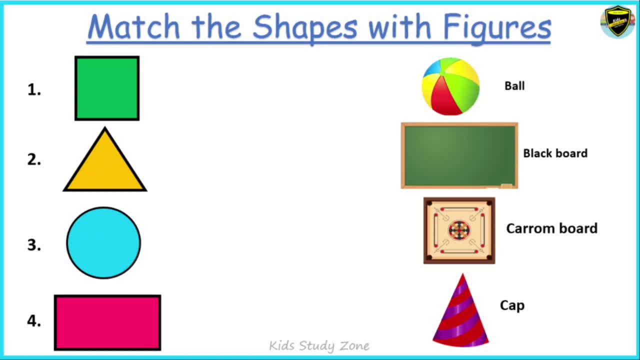 No, Is it a blackboard? No, Is it a carom board? Yes, The square shape matches with a carom board. Well done, children. Now let us see the next shape. This is a triangle. Now let us see the shape. triangle matches with which figure. 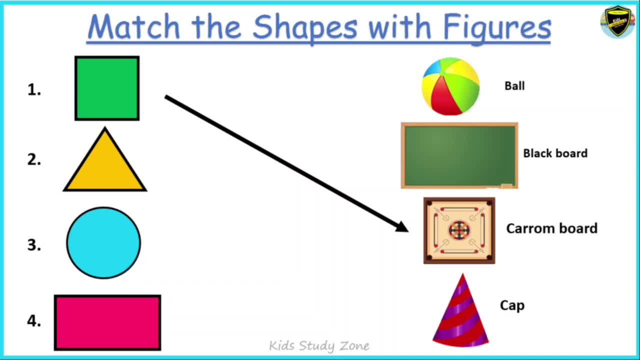 Now the options left are ball, blackboard and cap. So the shape triangle matches with cap. Very good, Now let us see shape number 3.. This is a circle. Now let us see from the remaining two options. 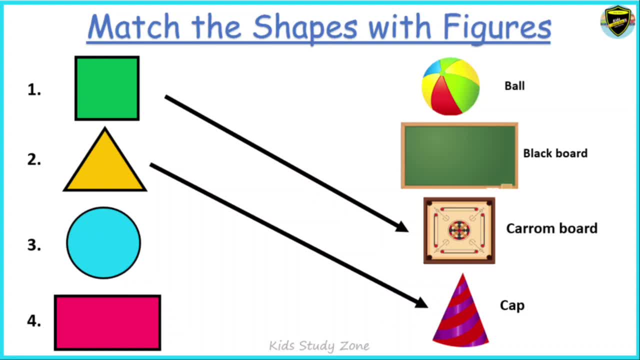 the shape circle matches with which figure? Is it a ball Or a blackboard? The shape circle matches with the figure ball. Very good, children. Now let us see the fourth shape. This is a rectangle, And the option left over here is blackboard. 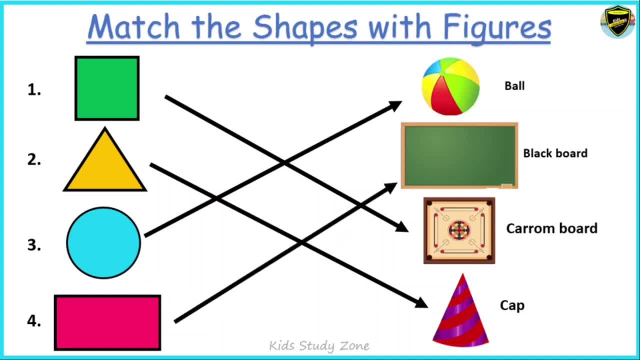 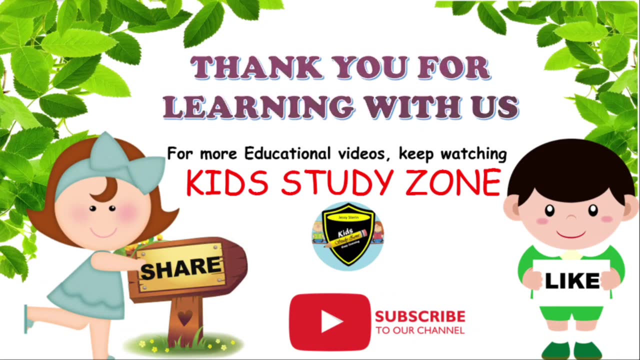 That's the right answer. I hope you learnt and understood about different shapes and you will remember this Whenever you are going to learn about shapes again. Thank you so much for learning with us. Keep watching KidStudyZone for more educational videos.